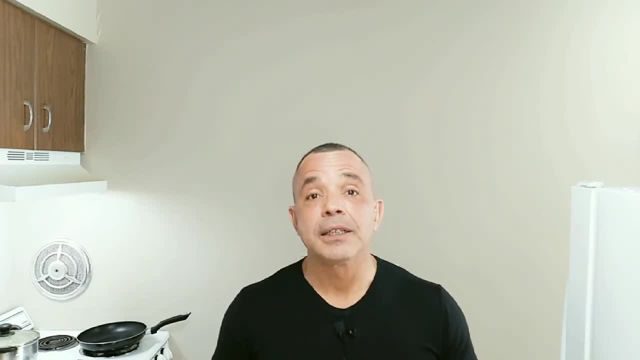 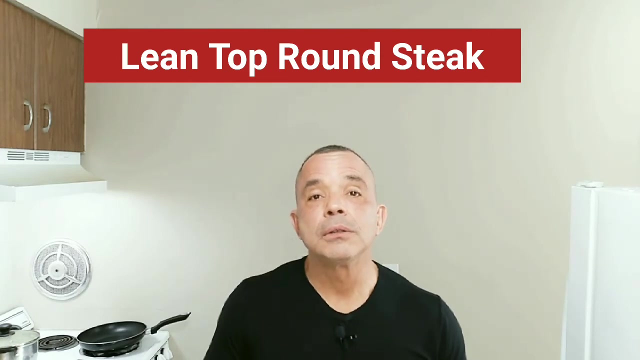 of protein. The best way, the only way, I feel, is to, if you're going to be using- I'll be using, for an example, the lean ground- excuse me, lean top round steak. First thing you do, you trim your fat. get rid of as much of the fat as you want. 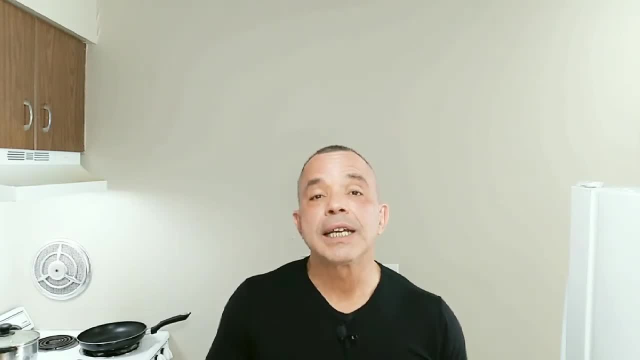 Top round is not very fat. That's the reason I like to use that as my steak of choice. So all you do is you trim your fat. Then what you'll do is you'll however you're going to cook it, you're going to grill it, pan fry it, broil it. whatever you're going to do. 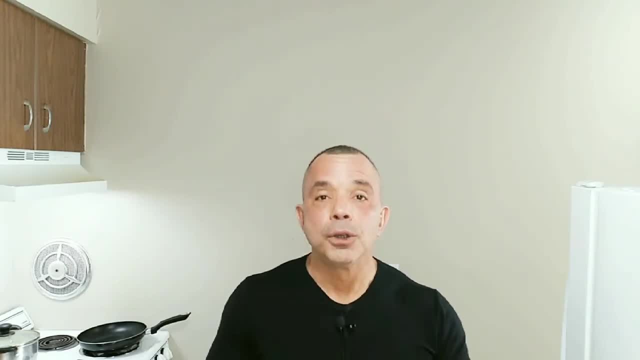 After it is cooked and it settles down, you pull it out of the oven, Then you cut it up into how many other pieces you need, put it on a scale and then that is going to represent how many grams of the cooked weight that you have Now from the grams of the cooked 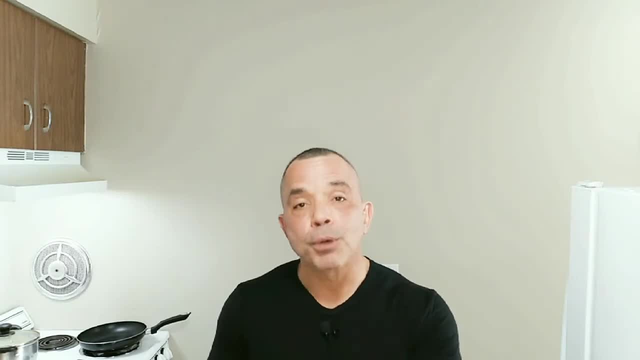 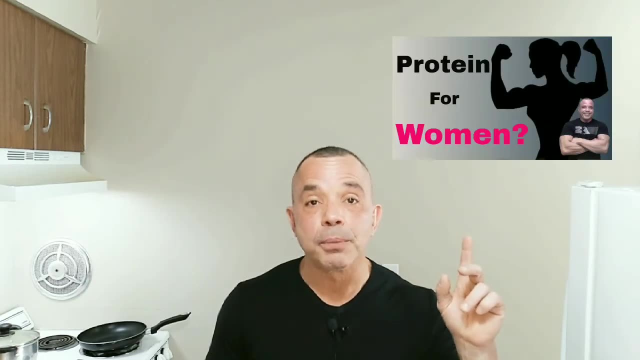 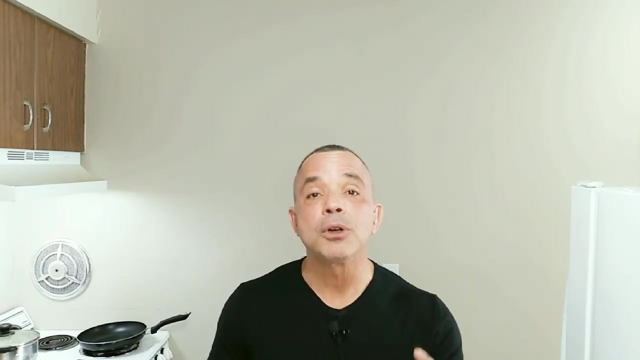 weight, you will have how many grams of protein is in the cooked weight. If you've seen any of my previous videos, this video right here will be definitely going to help you out. So, if you're- if you're a female, because it'll tell you how much protein you need for a female, but I'm going 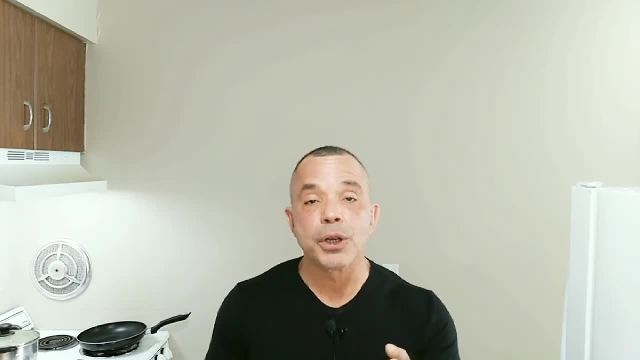 to put in the description the conversions for you. I'll put top round steak and I'll also put ground beef. So, speaking of ground beef, what you have to do is you have to cook your ground beef, You have to drain it. What I would do is I'd put it in a spaghetti strainer. 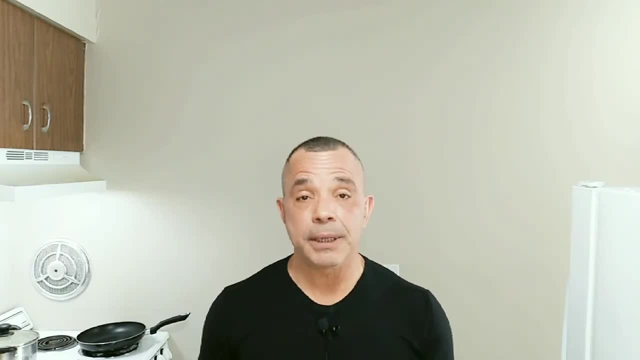 drain out all the water, all the juice, and then the same thing applies. If you have 100 grams of ground beef, you're going to put it in a spaghetti strainer, and then the same thing applies If you have 100 grams of cooked weight ground beef. that's not 100 grams of protein You need. 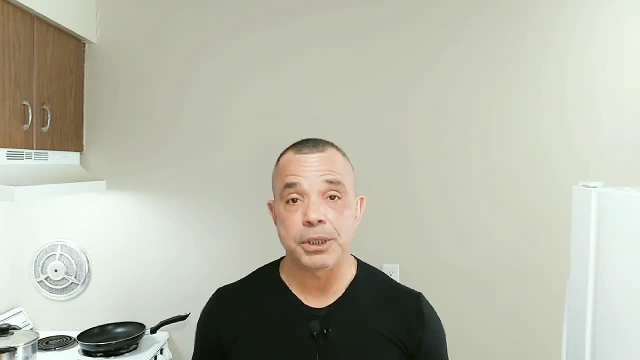 to consult the chart which I put in the description, making it very easy for you. So just remember, when you're weighing your stuff, you have to be precise. You cannot just guess. You have to be precise If you're serious about achieving your goals in terms of your nutrition. I can't.